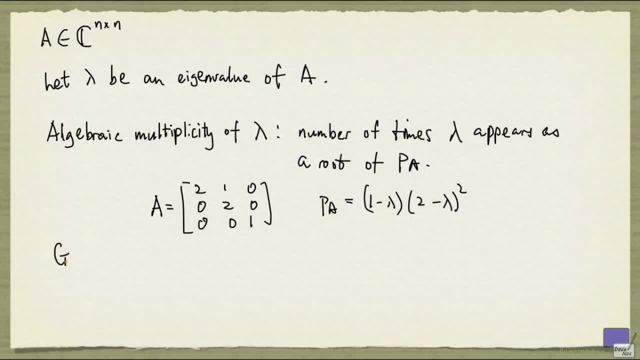 The algebraic multiplicity of lambda appears as a root of the characteristic polynomial 2 times, and the other quantity is called the geometric multiplicity. The geometric multiplicity is given by the dimension of the eigenspace for the eigenvalue lambda, And the eigenspace for the eigenvalue lambda will be denoted by: 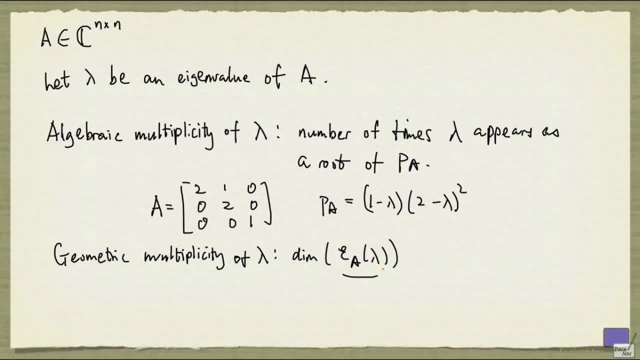 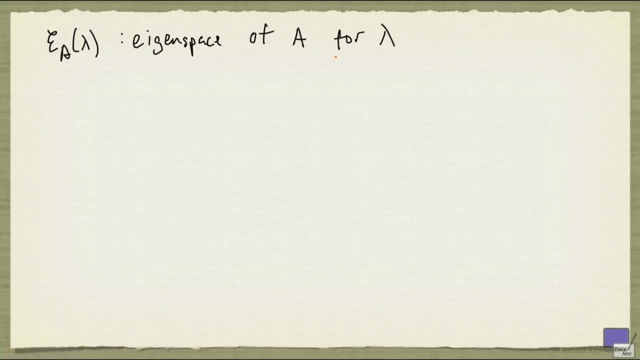 script E, subscript. A open bracket, lambda- close bracket. And we are now going to look at the definition of the eigenspace. So the eigenspace of A for lambda is given by the null space of the matrix, A minus lambda times the identity matrix. 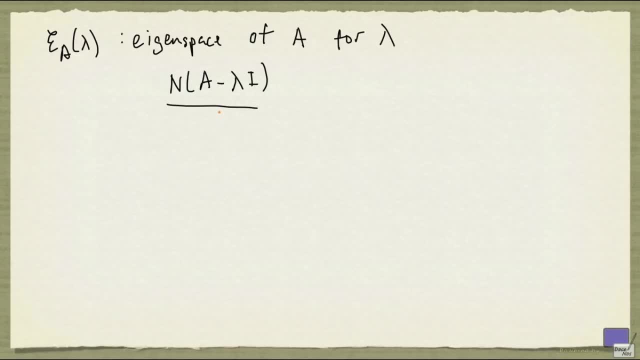 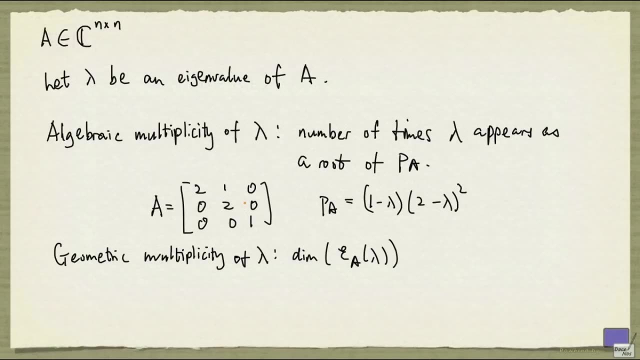 And remember that the non-zero vectors in the null space of A minus lambda I are precisely the eigenvectors of A with eigenvalue lambda. So let's go back to the matrix here and see what the geometric multiplicity of the eigenvalue 2 is. 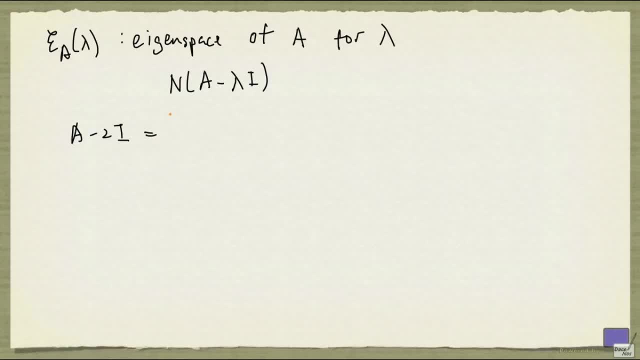 So we are looking at the null space of A minus 2 I, which is precisely 0, 1 0, 0, 0.. And 0, 0 minus 1.. And this matrix is rank 2.. So the dimension of the null space of A minus 2 I is 1.. 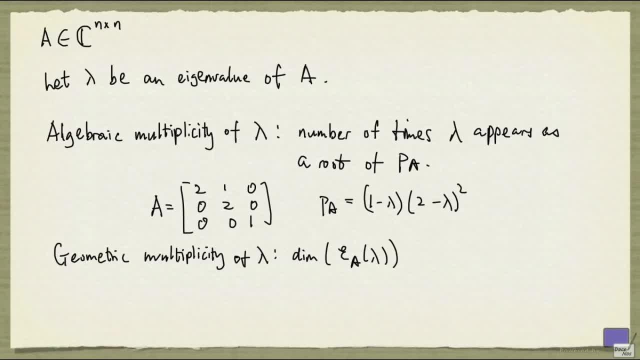 So what that means is the eigenvalue 2 has geometric multiplicity 1.. Notice that for the eigenvalue 2, the geometric multiplicity is less than the algebraic multiplicity And, in general, the geometric multiplicity of any eigenvalue. 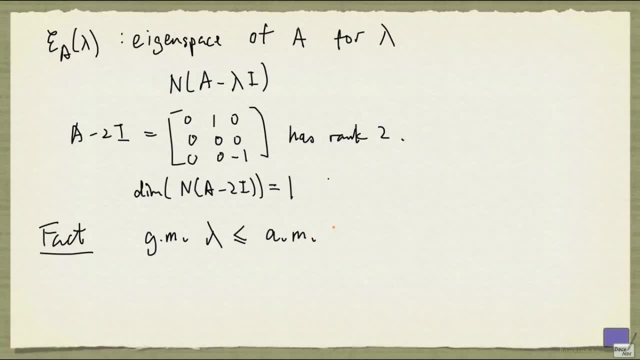 cannot exceed the algebraic multiplicity of the eigenvalue, And we have seen that in general this inequality can be strict. Now notice that if you have an eigenvalue that has algebraic multiplicity 1, then automatically its geometric multiplicity must be 1 as well. 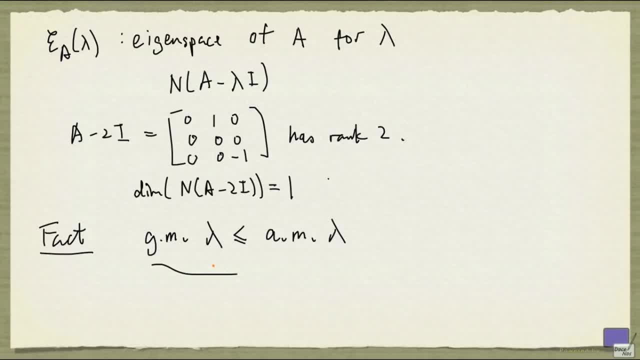 First of all, the geometric multiplicity of the eigenvalue cannot exceed 1 in this case, But it has to be at least 1 because by definition we must have a non-zero vector in the null space of A minus lambda I, And that means the rank of that matrix cannot be 4..